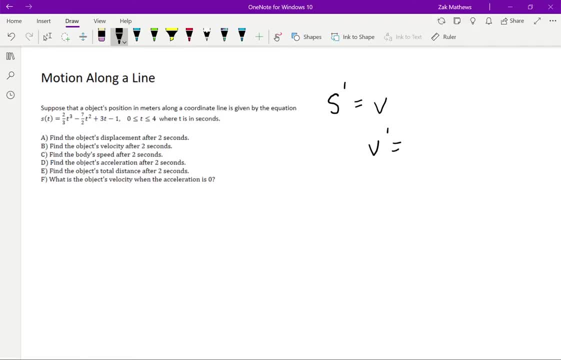 How quickly are we changing in speed? We look at the rate of change, of the rate of change or the change in speed. That is what's called acceleration, And we can continue to take these derivatives. We've talked about this a little bit in earlier videos, how we can continue to. 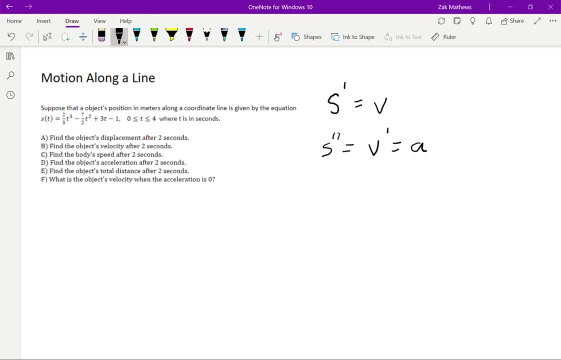 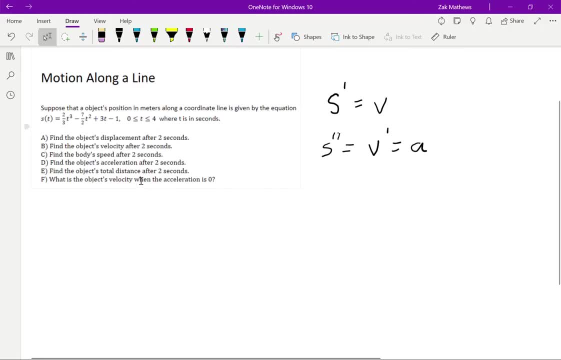 to remind ourselves of these ideas. We want to remind ourselves of these ideas, And these ideas are going to be very important in this problem. so let's look at what we need to be doing First. the was to find the object's displacement. 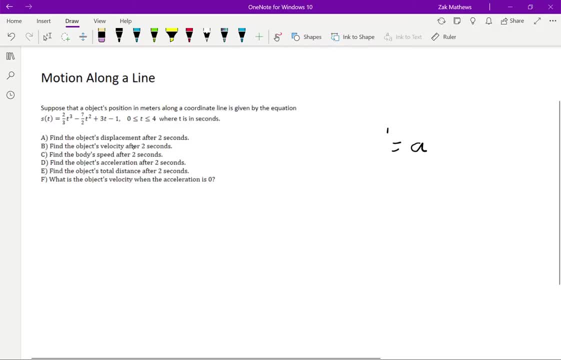 after two seconds, Let's talk about displacement versus distance. They sound very similar, but they're different. In order to talk about displacement versus distance, we really need to start up with the discussion of velocity – sorry, with vectors versus scalars. a vector takes into consideration direction. a scalar just looks at the total magnitude, so we 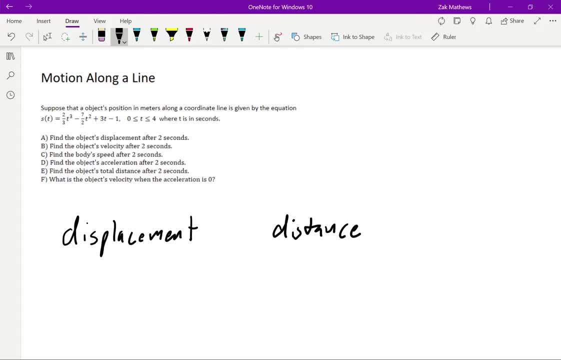 need to determine which of these is the vector and which of them is a scalar. the displacement. all it cares about is where we start compared to where we end up, and so it doesn't we, we, we care about how we are getting to that point, where we start versus where we end up. so if we take some 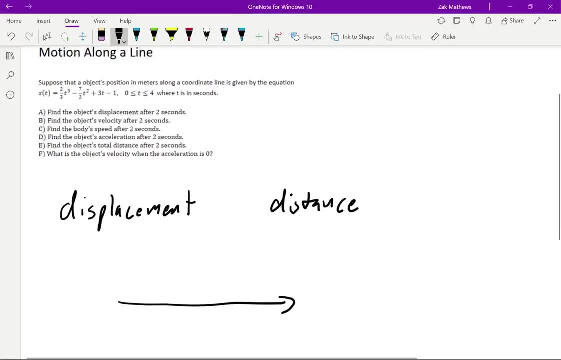 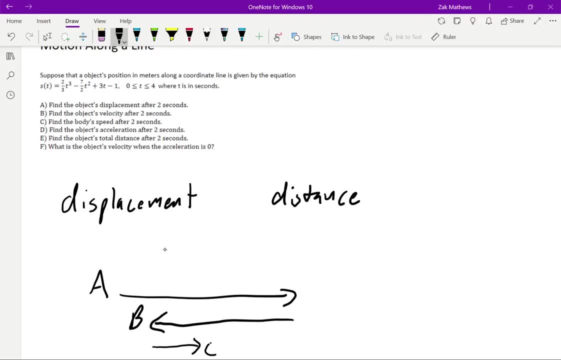 turns in there if we say come down this direction and then we turn back like this: to turn, I'll call this point a, point B and we come back up this direction. let's say a little bit, get to point C. the displacement is talking about from point a to point C, this red distance right in here. 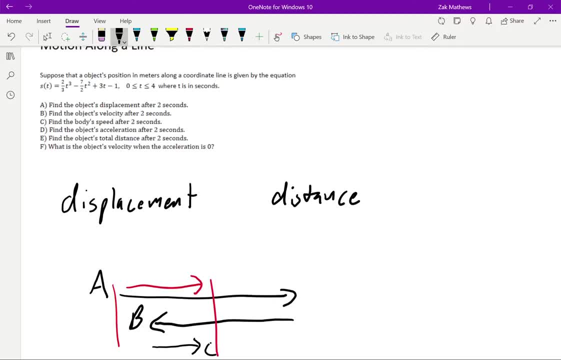 because we care about where we start and where we end. every turn along the way you take is important. that means that displacement is a vector. distance doesn't really care about those turns. all the distance looks like are those initial black lines, this distance here, plus this distance, here, plus this distance. so we are ignoring all of those turns. we're 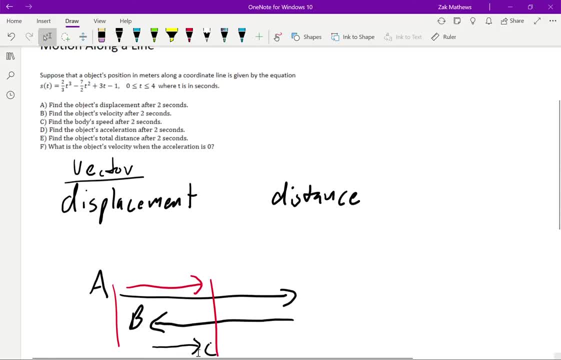 just looking at how far we've traveled along the way, and so, for that reason, distance is a scalar. vectors: we care about how we get there, what turns we've taken, displacement: we care about where we start, where we finish. so how we get there matters, scalars, we just 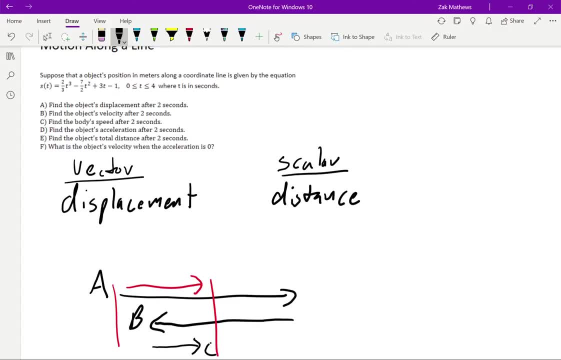 want to do that. total magnitude, other vectors versus scalars. velocity is a, is a vector, speed is a scalar. nice alliteration there. it makes it easy to remember. velocity cares about directions, can have a positive or a negative velocity. Positives moving forward, negatives moving. 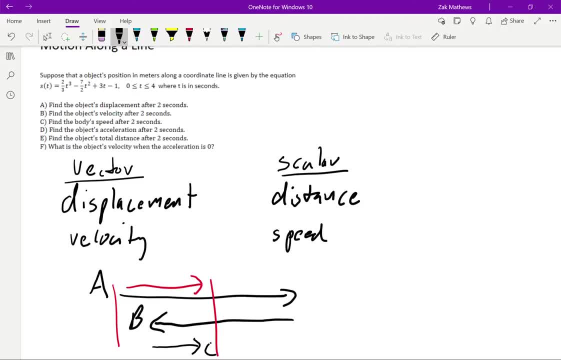 backwards Speed. all we care about is how fast we're going. We don't care about if we're going forwards or backwards, it's just the total speed. So keep these ideas in mind. So in this first problem, we're asked to find the displacement. This is the one that all we care about is how. 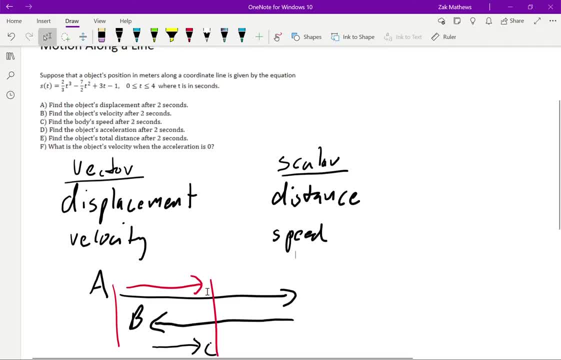 far we have traveled, from where we start to where we finish- Let me clear a little bit of room here- And so we have the equation that gives us the position. What I'm going to do is I'm going to calculate the position at zero seconds and I calculate the position at two seconds. 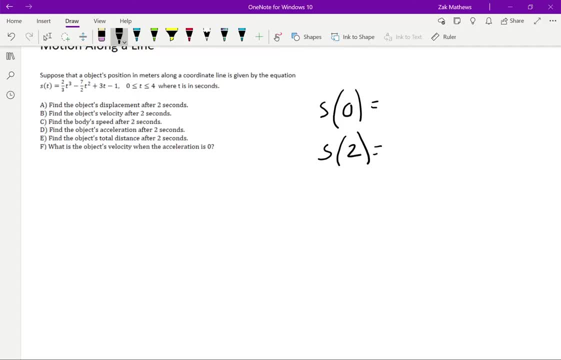 Why is it important to calculate the position at zero seconds? Well, that is my starting point. T is equal to zero is always my starting point. I don't necessarily start at zero. Sometimes we could be measuring from a different object, So maybe you know if this is my house and 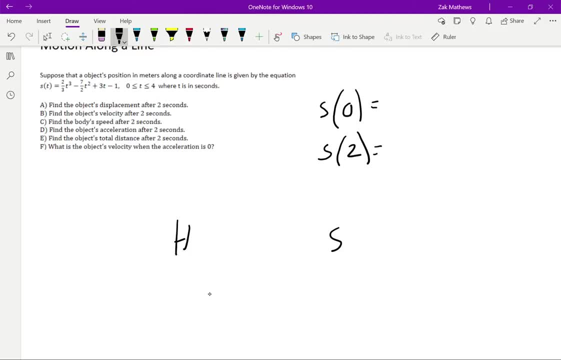 I'm starting off here. maybe I want my house to represent position zero because it gives me a good frame of reference. So if I start here, maybe I go back home and I go off to work and then I go somewhere else. I'm using that house as a central frame, So don't assume that the position at time 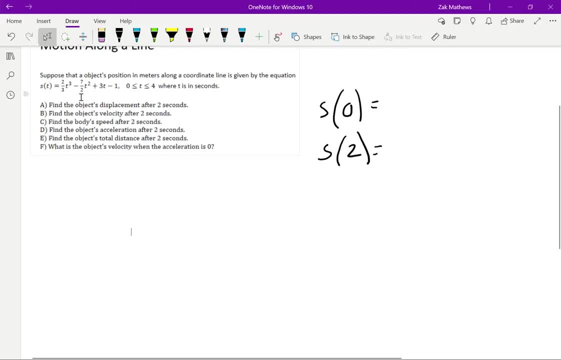 zero is equal to zero. We need to calculate this. We're going to do it just by plugging into this equation. So we'll have two thirds times zero cubed by seven halves times zero, squared plus three times zero minus one. So if we add all these together we get negative one. 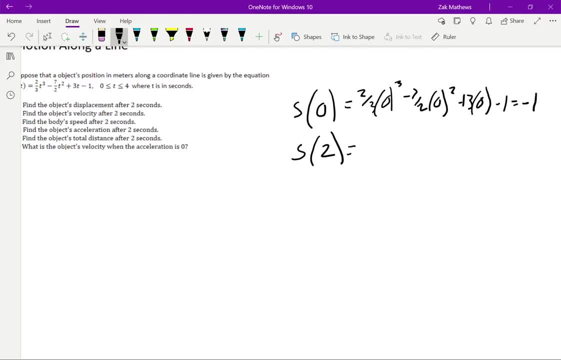 Slide over a little bit negative one. I do the exact same thing for the two. So we're going to have two thirds two cubed by seven halves times two squared plus three times two minus one. So I'm going to pull out my calculator just to speed me up a little bit through this process. 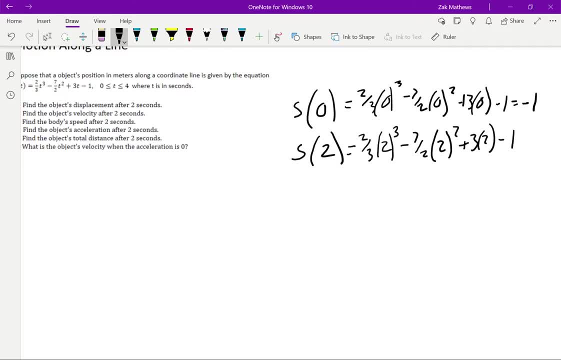 I have two over three Times two. cubed is eight minus seven halves. Seven halves times two. squared is four plus six minus one. So if we add up all those and convert this over to fraction we get negative 11 over three. So if we were to kind of view this, 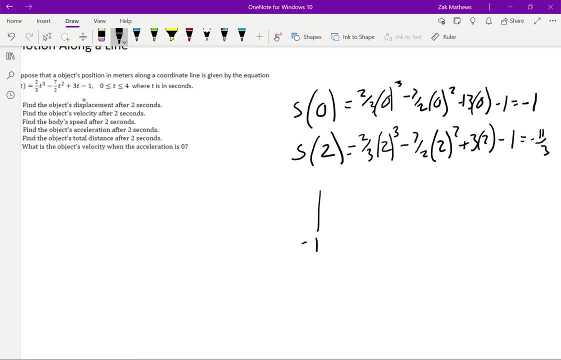 on the number line at t is equal to zero, we are starting at a position of negative one. From there, we are actually going backwards To a position of negative 11 thirds. To calculate this displacement, we always take wherever we ended up, negative 11 thirds in this case. 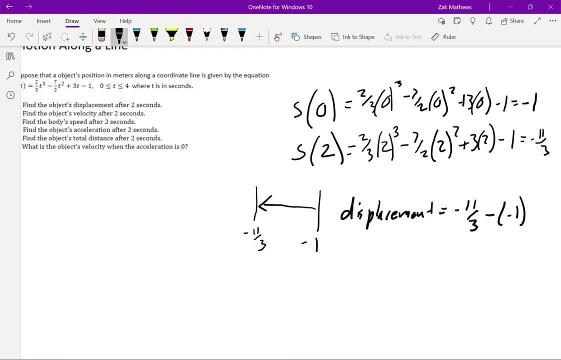 we subtract wherever we start. So displacement. just write out an equation for this: Displacement is equal to the terminal position minus the initial position, Initial position. The order matters with displacement. The order matters because it takes into consideration direction We care about. are we forwards of where we were or are? 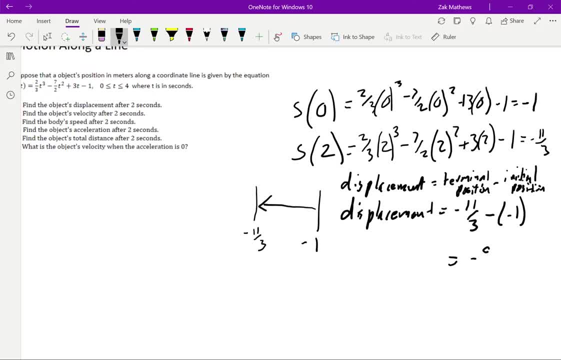 we backward, In this case we get a total displacement of negative eight thirds. That means that we have traveled backwards to get to this location. If we think about our units- Negative eight thirds meters. we have traveled backwards by two and two-thirds or eight-thirds meters to get to this terminal. 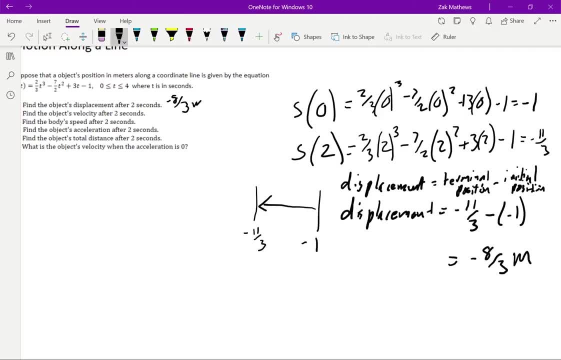 position. So I'm going to just kind of keep track of these answers as I go along. that way we can talk about them. All right. so negative eight-thirds is our answer for A and I might have to erase this again just so I can see my problem. so it can be just a second to erase The problem number. 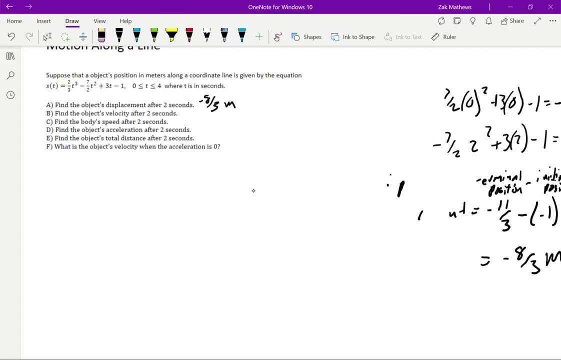 or letter B, rather find the object's velocity after two seconds. All right, so now we need to know velocity. Remember what we discussed at the beginning: velocity is simply the derivative of the position equation. So let me go ahead and calculate the derivative of the position equation. 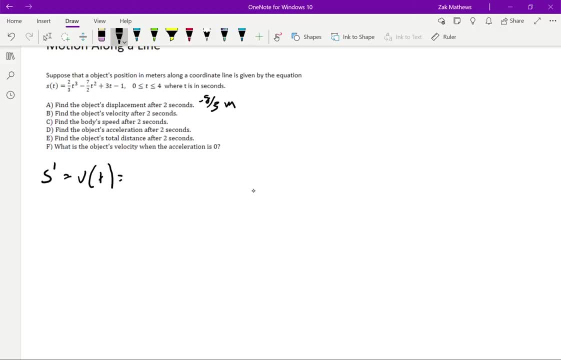 which does give us velocity at time. t. We multiply the three to the front, we get two t squared. Multiply the two to the front of the next term, right here, and we get minus seven t And the derivative of three t is just three. Derivative of one is zero. So there is my 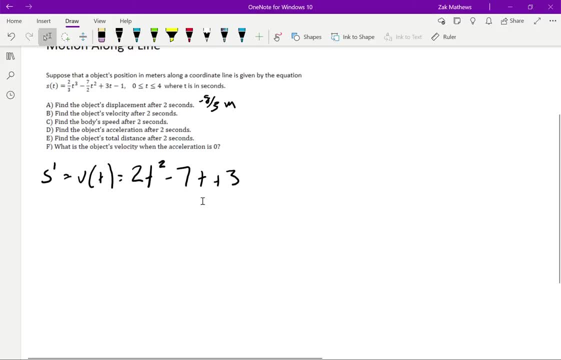 derivative of three t Velocity. for this problem I want to know in B what is the object's velocity after two seconds. So I'm going to plug this two into my new equation. So we'd have eight minus fourteen plus three negative. six plus three would give us negative. 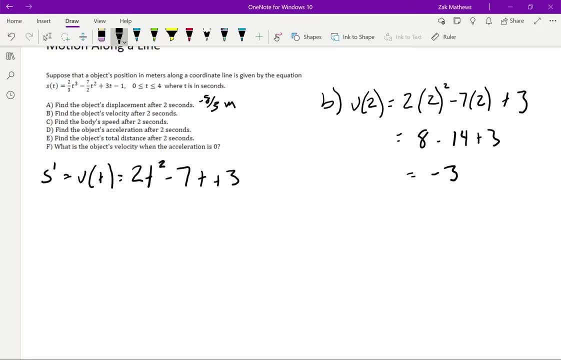 three Velocity. what is our unit on this? Well, we probably know from just speeds: we travel in miles per hour, meters per second, whatever the situation would be. And here we do have meters per second. We think about why that is. It is a rate of change, We are 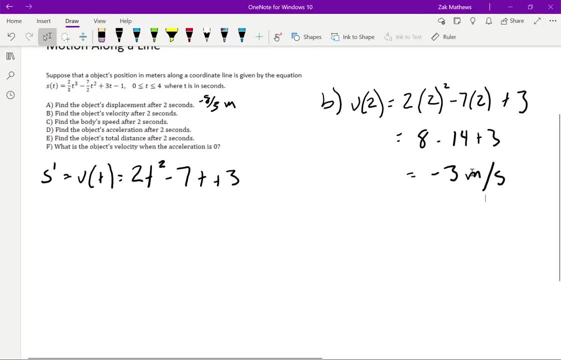 changing the distance, the meters, over a certain amount of time. So that's where we're getting the meters per second. So for B we get negative three meters per second. Go ahead and clear off some room for the letter C, And so all these calculations. I just keep raising This. 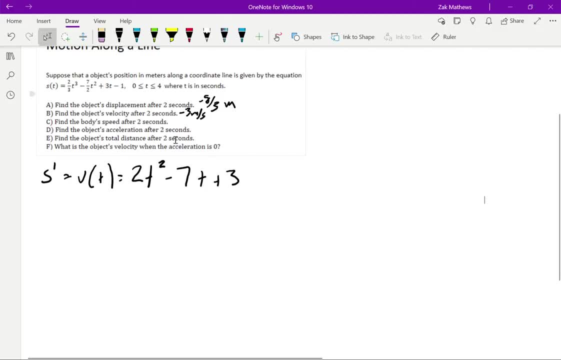 would be what I'd expect to see on your paper. It's just so that we can look at the problem at the same time. I'm erasing it, But if I asked you to do a problem like this on your paper, you would just have all these calculations worked out on your paper. All right, letter C: Find the. 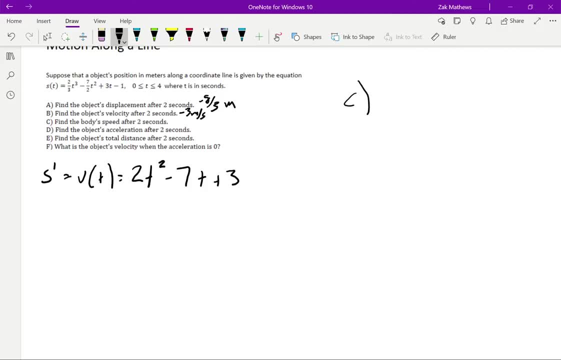 body's speed after two seconds. Well, it's actually going to be that thin calculation. we just did right. We found the velocity equation, We plugged in the two seconds. We got a velocity of negative three meters per second. But speed is just the scalar of that. 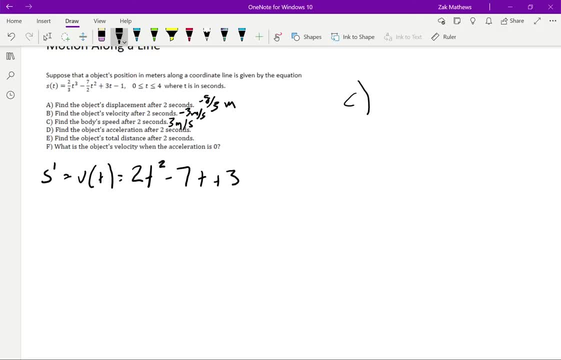 And so it's going to be the absolute value. It's going to be the positive. Speed is always a positive. It doesn't care about direction. Could velocity and speed actually be the exact same answer? Yes, they could. If our velocity was positive, it's traveling in that positive. 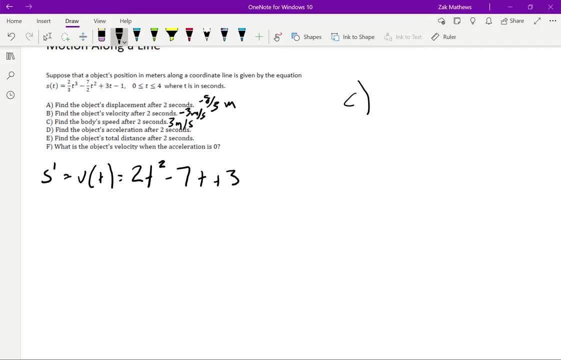 direction They will be exactly the same. But if the velocity is negative, we need to make the speed positive. Speed always has to be a positive. All right, letter D, That one didn't require any work. Letter D: Find the object's acceleration after two seconds. Well, if I need to know the. 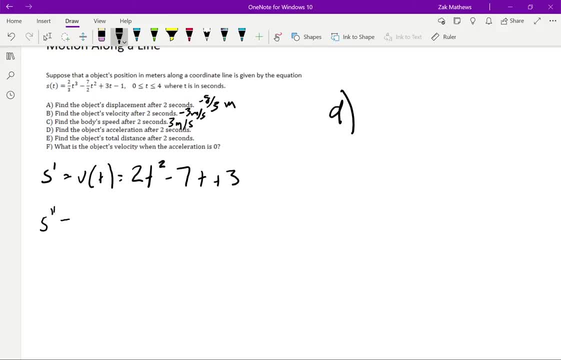 acceleration I need the second derivative or the first derivative velocity. So we multiply the two to the front, We get four t minus seven. So there's our acceleration equation. Acceleration based on time t is equal to four t minus seven. I want to know the acceleration after two seconds. 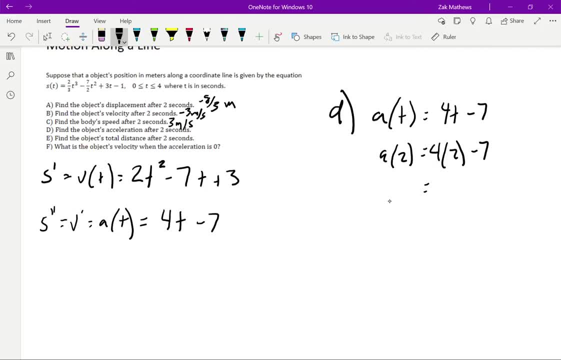 so I'm going to plug that two in. Four times two is eight minus seven gives me one. Our unit on this is one. Well, velocity was meters per second, and now we're looking at another rate of change, So meters per second, per second, which that looks really goofy. How we'd write that is meters per 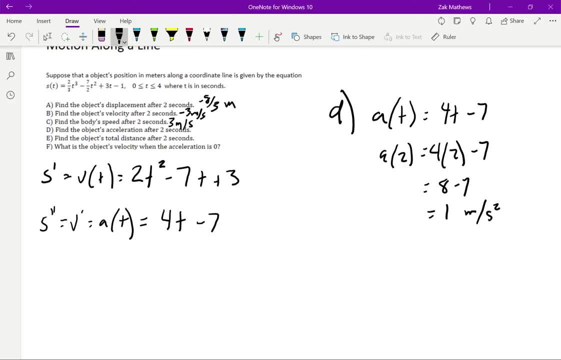 second squared. Acceleration is always measured in your distance measurement divided by your time measurement, squared. And so for letter D we get one meter per second squared. Acceleration is a vector, So you will always keep it sign with it. It does matter if you're accelerating versus. 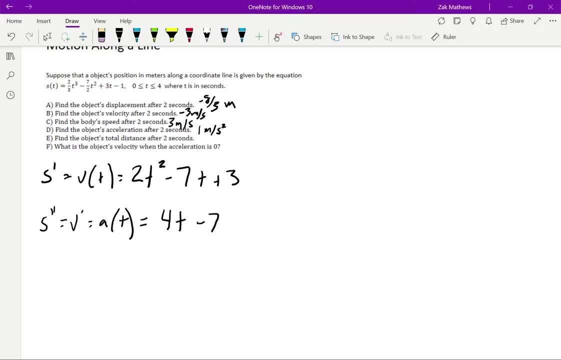 decelerating. There's not like a speed equivalent of acceleration. If you're asked for the magnitude of the acceleration, if you want to know just the absolute value of it, you'd be asked for exactly that was the magnitude of the acceleration. All right, let's move on to letter E. This is going. 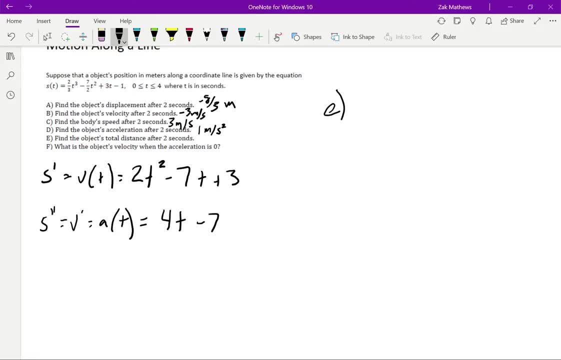 to be the most work of any that we've done to this point. Find the object's total distance after two seconds. So just a reminder. how is this different than A Distance? we care about all those turning points. So if I travel, 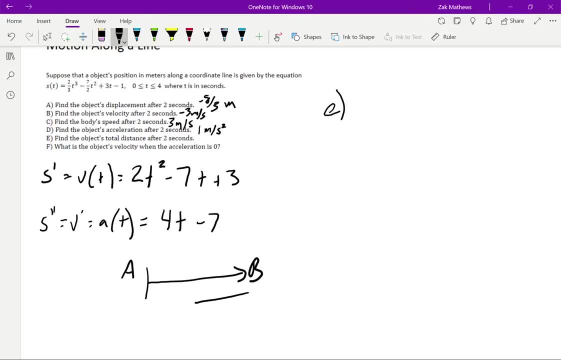 from A to B and then turn and then go back to C and then turn and then go up to D. I would need to add up all these little line segments here. I need to know all those line segments rather than just saying I've gone from A to D here. Another way to think about this is think about a runner running. 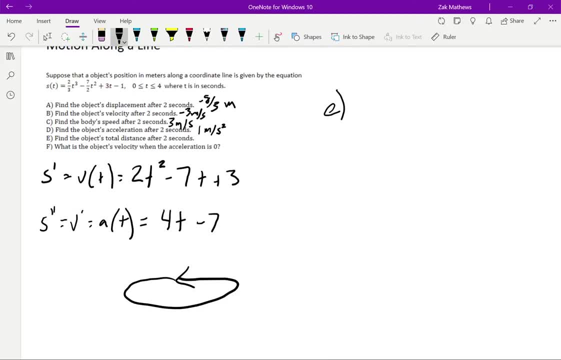 around a track. I always like to check this as one of the most pointless activities because once you finish, once you complete, however many laps you're going to do- you started here, you end right here. Once you finish, your displacement is zero. You can run all day long and you have a displacement. 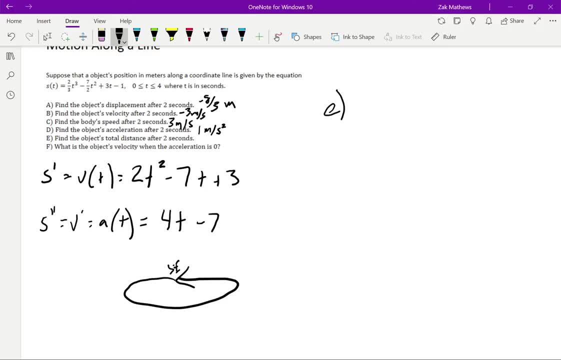 of zero. Of course, that's not what a runner would want to measure, right? A runner wants to measure: how far did I travel in my journey? Not the displacement, but the distance, And so they're adding up. well, I traveled 400 meters, around, 400 more, 400 more. They're adding up. however, 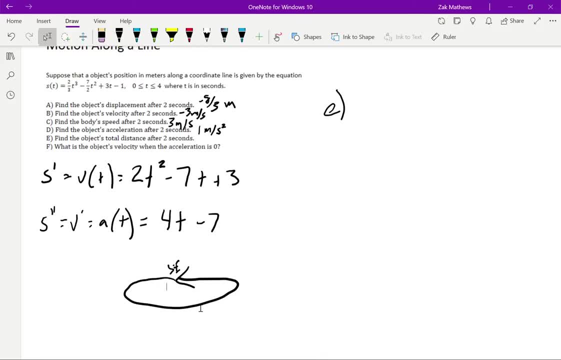 many laps that they've done. So that's what we need to do here: We need to figure out where did we turn. How far did we go between turns? Well, we don't know where we turned yet. We're gonna have to start with that. Let's think about when we're turning. Just if you would demonstrate. 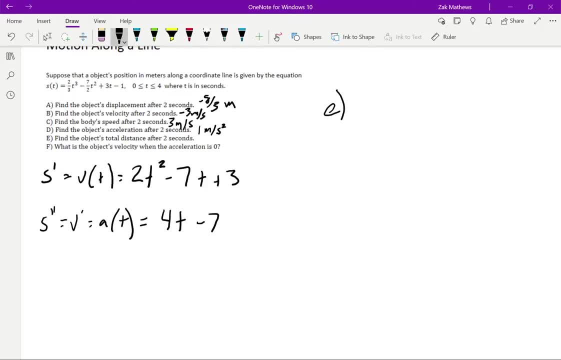 this yourself? I would. I would literally just walk around the classroom to show you this. Let's say, we start walking and I want to turn the opposite direction. At that instant in time, I have to come to a complete stop. That's the only way I'm going to turn. I have to come to a complete 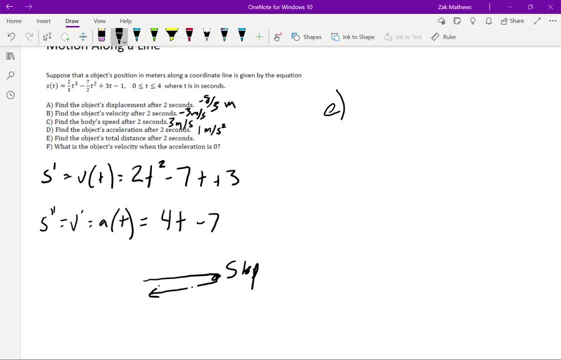 stop. so what that means is the turns will have to occur when the velocity is equal to zero. turning points must occur when your velocity is equal to zero. now are all points where the velocity is equal to zero a turning point. that is also not true if you think about coming up to a. 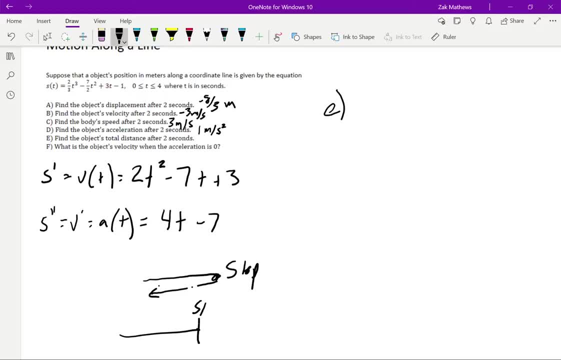 stop sign. you're driving along, you stop at the stop sign and then you keep going. well, you stopped there, you kept going and that is not a turning point. so we need to be careful that when we are looking at when the velocity is equal to zero, those are potential turning points. so let's look. 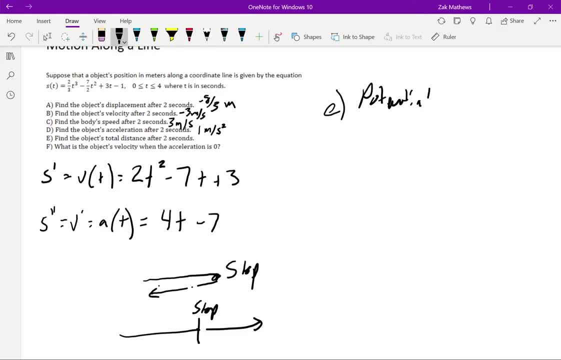 for those potential turning points first, and we'll talk about how to determine if they are turning points or not. all right, so i'm going to. that's a point that's a little hard to read. i set my velocity equal to zero. remember the velocity equation was a two t squared. 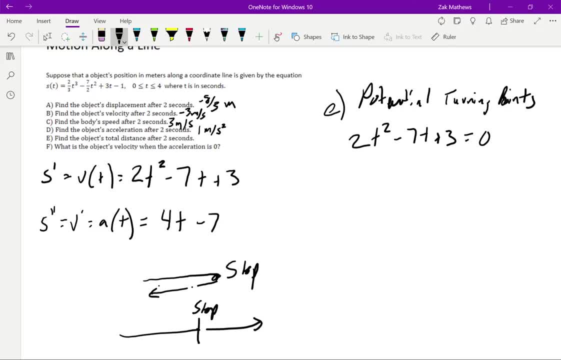 minus seven, t plus three. i set that equal to zero. this is a quadratic, so i can factor it. we would always want to. anytime we have a non-linear equation, we want to factor it in some way. we can use a rational zero's theorem, we can use synthetic division. in this case it is just. 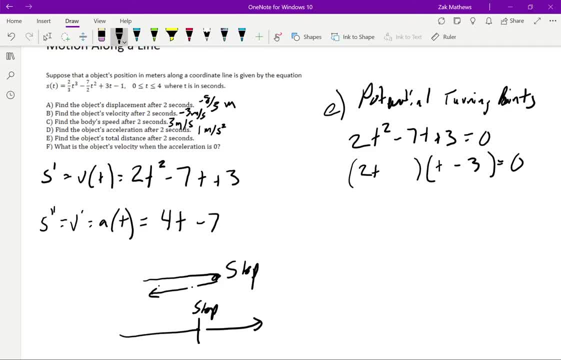 quadratic, so i can factor as two t and t. it's going to have to be a minus three and a minus one. so i get t is equal to one half. i get t is equal to three. so then the question is, are these actually turning points? now, if i'm finding the distance it really doesn't matter, because i can always 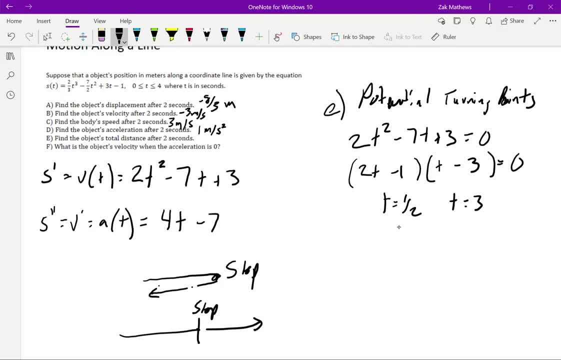 break up a line segment to sort of figure out what's going on, and then i can actually calculate the distance for smaller chunks, for instance in this bottom picture right down here when i'm coming up to the stop sign, continuing and then stopping again, or you know, just looking. 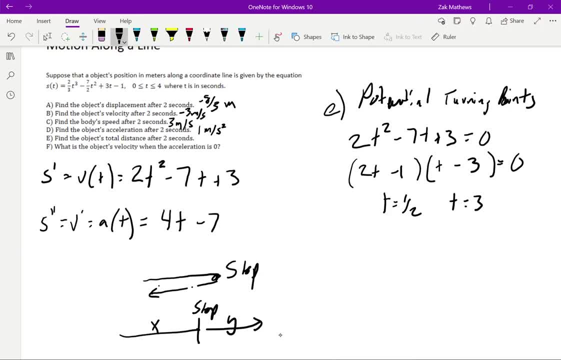 at terminal position. i can take x and y and add them together and that would be the same as just adding the whole initial length, z. where we want to be careful is in this first case, where i turned around, we undid all of that displacement. the distances were subtracting in the displacement. 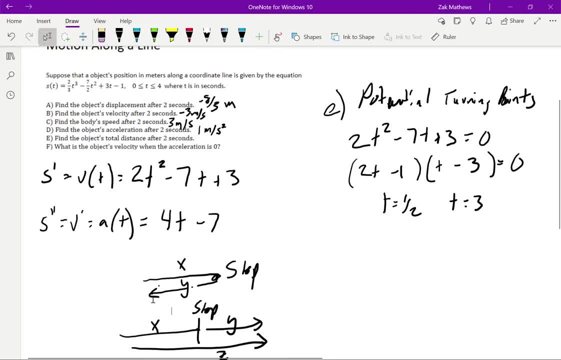 so we got back to where we started, like with our track runner, but we have two different amounts here that we need to add for the distance. so again, my point in all this: even if they aren't turning points, we can always break up the interval around these points. 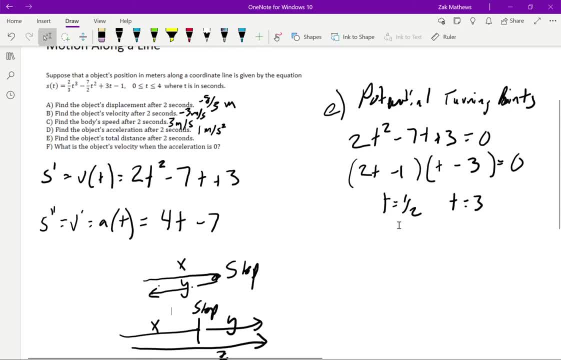 and that's just gonna. it'll be more work than necessary, but it won't hurt us if we're explicitly asked for turning points i need to think about: are these actually turning points? the answer to this is yes, these are both turning points. we have turning points. 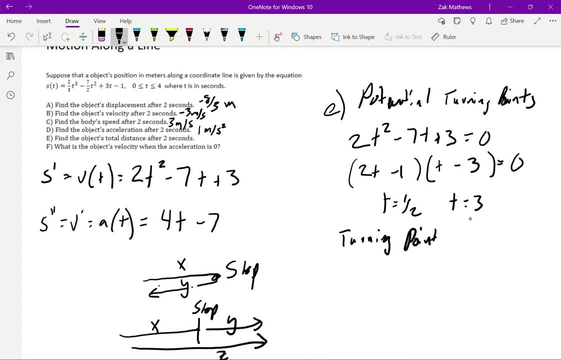 at t is equal to one one half, and then we're going to add the distance to the distance: one half and t is equal to three. now how could i check that? well, what we should see if they are turning points is that the velocity is changing sides signs around them. so, for instance, if we 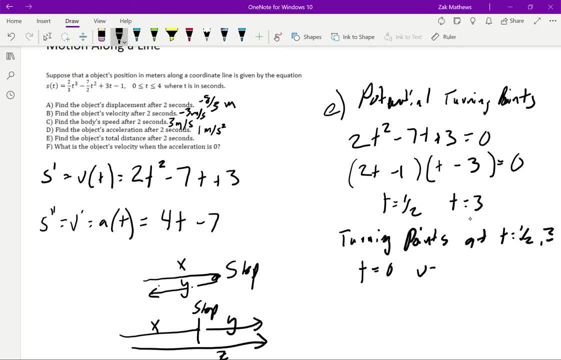 have, t is equal to zero. we should see that the velocity, if it's positive or negative, is the opposite, as t is equal to one and then t is equal to four. we better see those velocities change. so let's just plug these in real quick to prove these are turning points. take our zero, we plug it into. 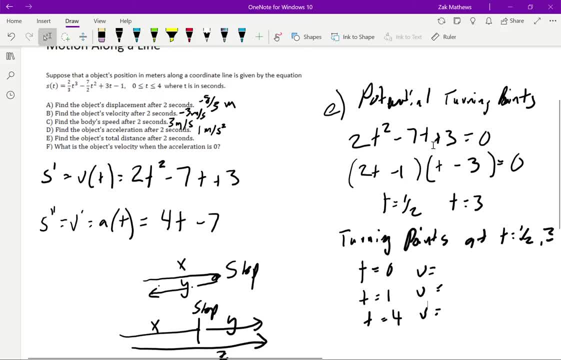 our velocity equation, this equation right here at the top. so it had zero minus zero plus three, that's three. that means we're moving forward. then we plug in our one. we'd have two minus seven plus three. that's negative two: the velocity is now negative. negative that means that we are traveling. 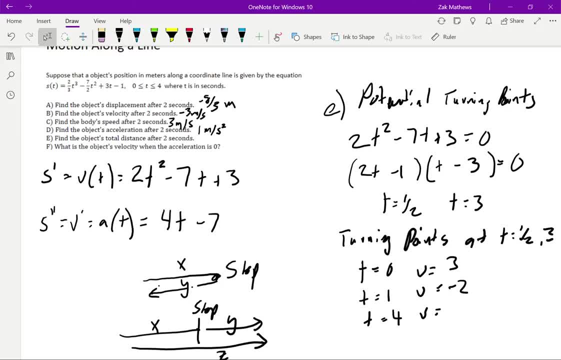 backwards. we have definitely turned inside of that interval. and then, finally, if we take the four, four squared is 16, double it is 32, minus 28 is four, and then add three more. if i did all that real quick in my head, it's seven. but again, the important thing there is that we have a positive and that is. 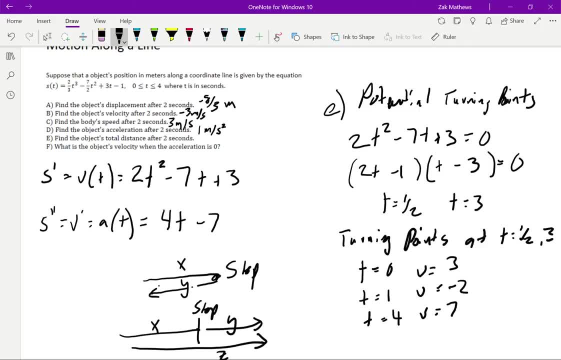 telling us that we are traveling forward, and so we can see that the one-third and the three must be turning points, because we saw that the velocities are changing signs from a positive to negative, to a positive. why is it that these have to be the turning points? well, they're the only places that the 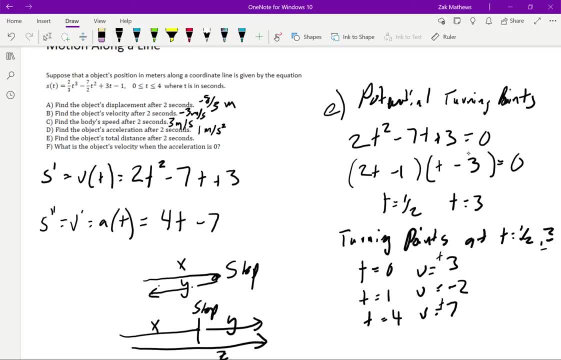 velocity was equal to zero. these are the only possibilities. so we definitely have turning points now. i did a lot of work there to prove something i could have actually determined very quickly. if you remember what polynomial functions look like, you remember some facts about their zeros. if a zeros or a x-intercept, a roots multiplicity, is odd. 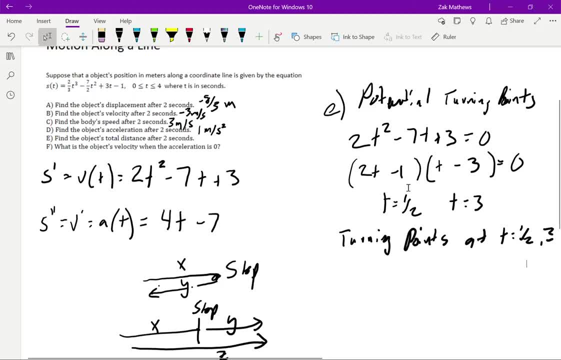 that polynomial will pass through the x-axis at that point, meaning it would change. i think about passing through the x-axis. it's changing from negative to positive either way. that is true for odd multiplicities. if we have an even multiplicity, it touches and turns. notice that both of these ends stay positive. so if we look at these, 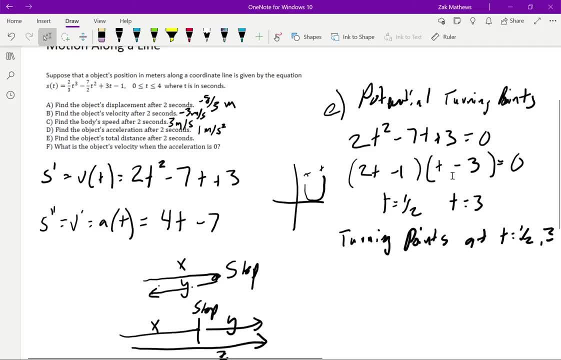 factors. both of these factors occurred once, meaning their multiplicity was just one, and that means they have to cross through the axis, meaning that they will both be turning points. okay, so that is how we can determine turning points for a motion along curve, motion along a line. 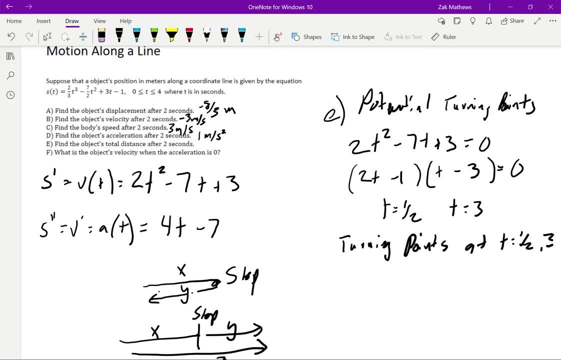 now that i have turning points, i'm still not done with the problem. right? i was asked for the total distance, and so how does this help me? well, we're going to need to know the position at 0. we're going to need to know the position at at the two. still right, those are still important. 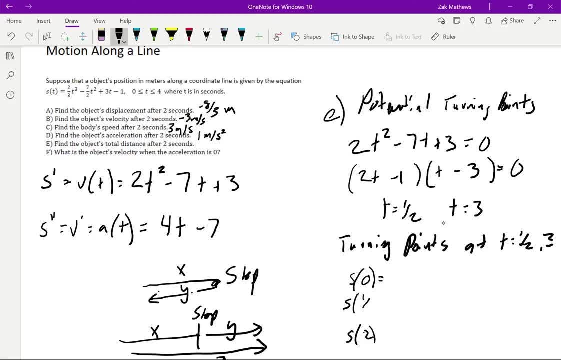 but i also need to know this position at one half, because this is again this top example here where i've gone a certain amount of distance, i turn, i've come back, i've erased the displacement, i've i've reduced the displacement, but the distance i need to. 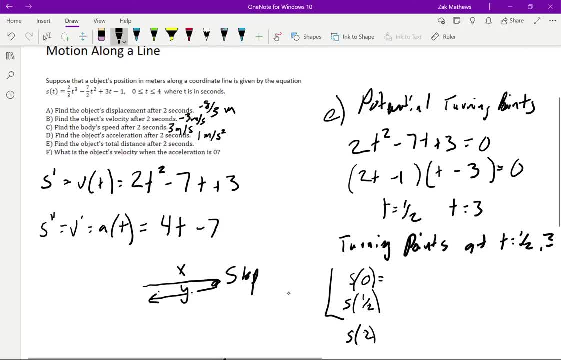 add both of these chunks. so i need to figure out how far did i travel here and then how far did i travel here. that's what i'm looking for. i'm going to essentially take displacements over both of these intervals. all right, so we're going to plug in. i'm going to do this a little bit faster, just. 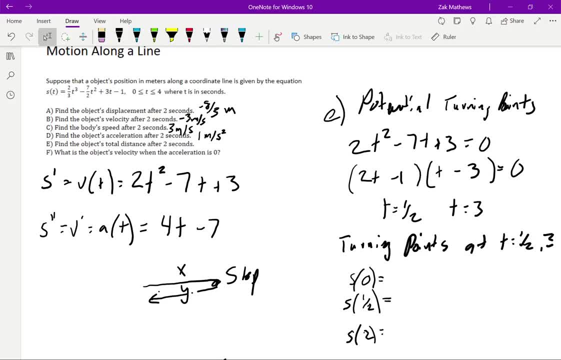 do it in my calculator to speed us up a little bit. so i'm going to plug in my zero first. well, this one's pretty easy, because we had it at the start. it was just the negative one. so the, the, the distance or, excuse me, the position at zero is equal to negative one. then i'm going to plug in my. 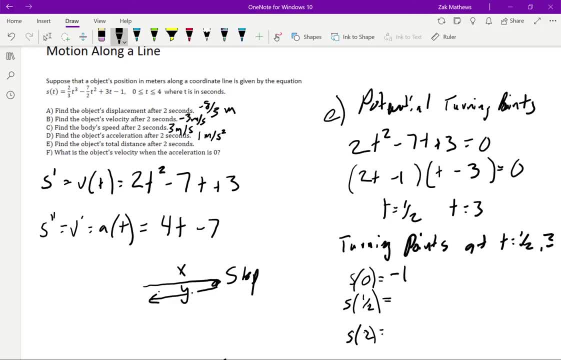 half. this is the one that we haven't done yet. um, let me just start by writing down my answer for s of two before i leave that, because i erased it from my page. this is one of the downsides to not having in front of us. it should be negative. 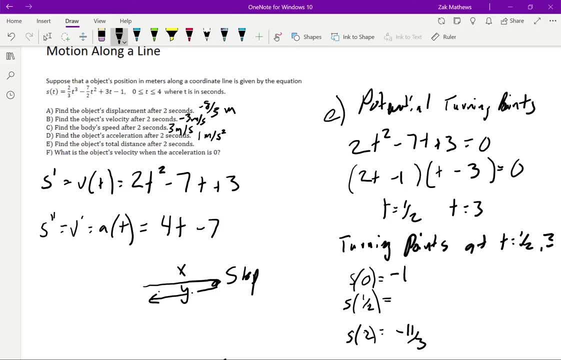 eleven thirds? yeah, that'd be right. all right, and now i'm going to type in my um my equation, with the one half plugged in, so we'd have two thirds and then we'd have our one half to the third third power. notice, here i'm plugging these into the initial equation. why is that? we want to know the distance. 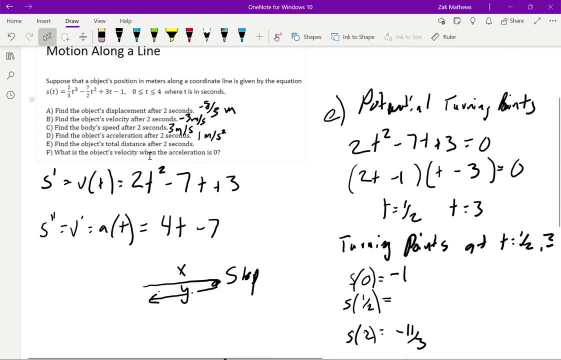 the distance is related to the position. we're plugging into the position equation, not the velocity. we know that the velocity at these points would be equal to zero. that's not what we're looking for. we want to know the position at these times. so we have the two thirds times one half. 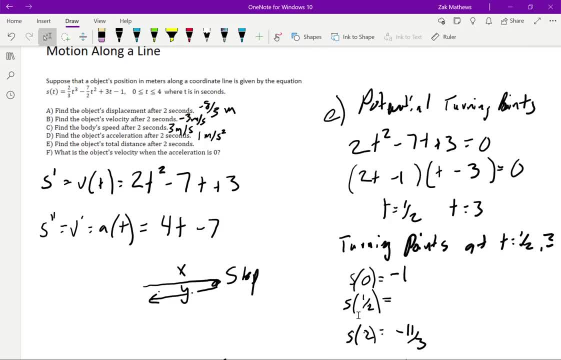 to the third power minus seven halves times one half to the second power plus three times the one half and then minus the one. so if we do all that, we should get an answer of right. uh, should be negative seven over 24.. so these positions are just that, they're just positions. we still need to know how. 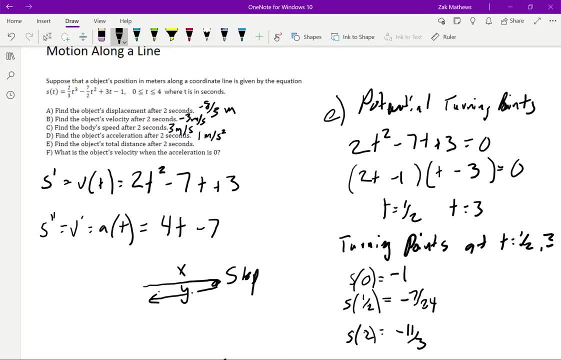 far we've traveled between each one. so i'm looking at what was my displacement here? what was my displacement here? really, i don't care about displacement. that's not quite accurate. i care about the distance between each um. we're going to do the same kind of. 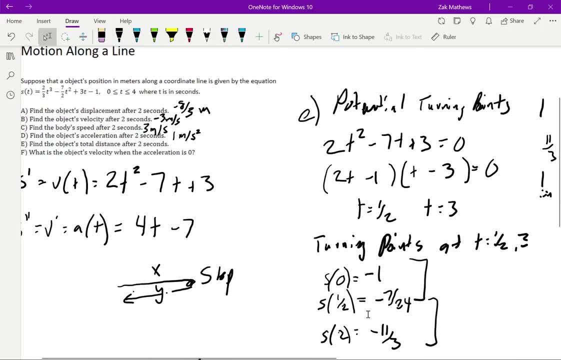 calculation as this, the displacement. but i'm going to make it positive. so i'm going to take the negative 7 over 24. i'm going to subtract the negative 1, the final position minus the initial. so if i subtract the negative 1 from this, i get 17 over 24.. then i take the negative 11 thirds. i'm 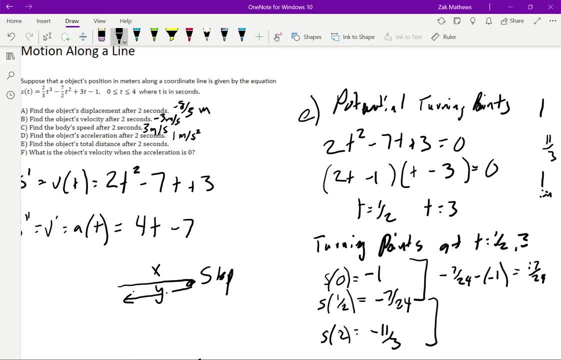 going to subtract the 7 over 24 from that and when we do that we should get a negative. uh, let me write it out: negative 11 thirds minus the negative 7 over 24.. we get a negative 27 over 8.. again, i don't need the negative, i don't want to use a negative. so 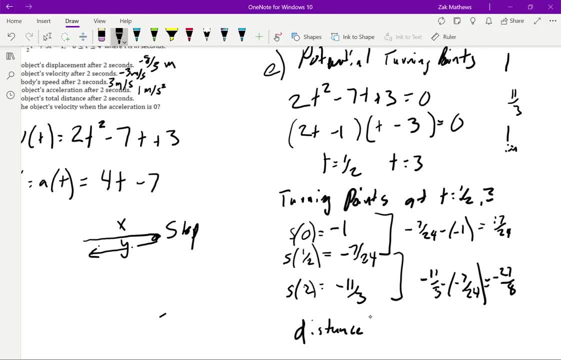 for my distance. what i'm going to do is i'm going to add each of these little little distances right, the I've gone in each tract, so 17 over 24 plus the 27 over 8. I'm just adding the positive version of that, and so when we add these two things together, we get 49. 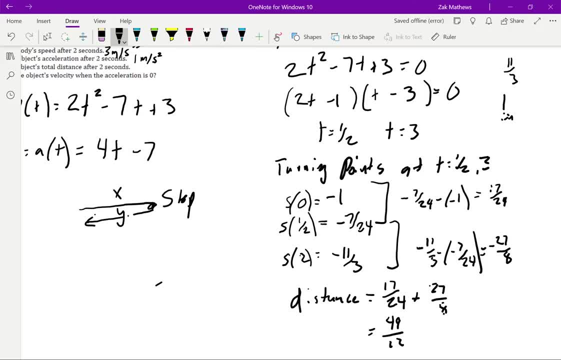 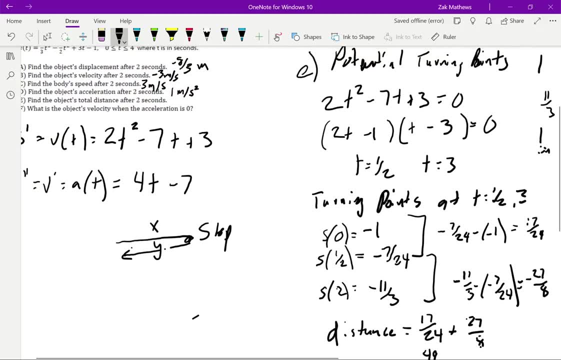 over 12, and so that is our total distance. we need to make sure that we are always including units, and so this would be 49 over 12 meters. be a little sloppy with this drawing arrow. 49 over 12 meters, so that one was a much larger. 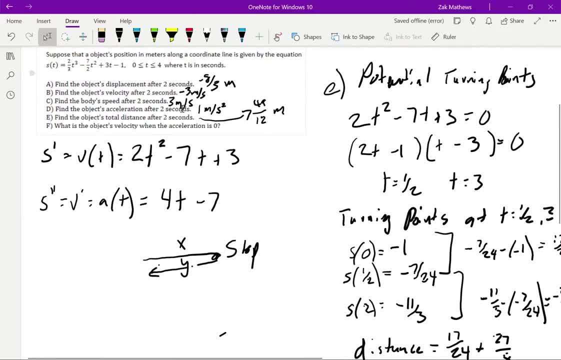 problem, or longer problem than the earlier ones. if we want to figure out that total distance, we have to know where the object turns. we weren't asked for that at the start, so we define those turning points first. how do we do that? we set the velocity equal to zero when we stop. those may or may not be turning. 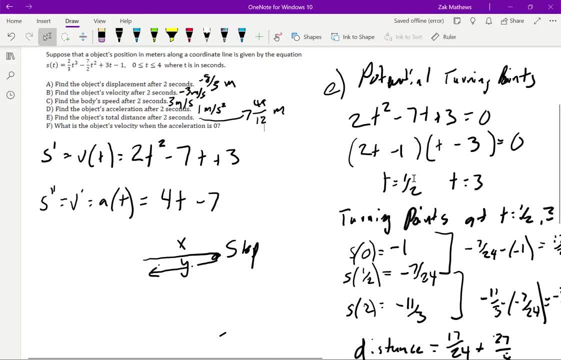 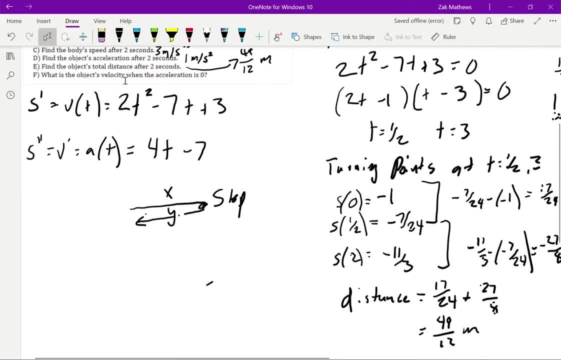 points. we've then got to determine that using the multiplicities or by looking at the sign of the velocity on either side of the turning points. once we know that something is a turning point, we were looking at the interval. we're going from 0 to 2. we're looking at the distance to 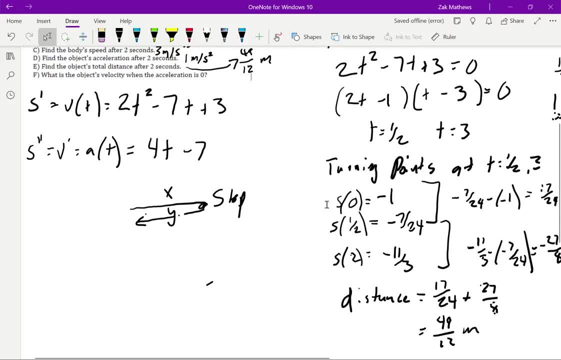 2 seconds. we're going to from 0 to 2, but we are stopping at one half, or we're kind of looking at how far we've gone after one half of a second, so we can add up all of those distances, all right, finally, what is the objects velocity? 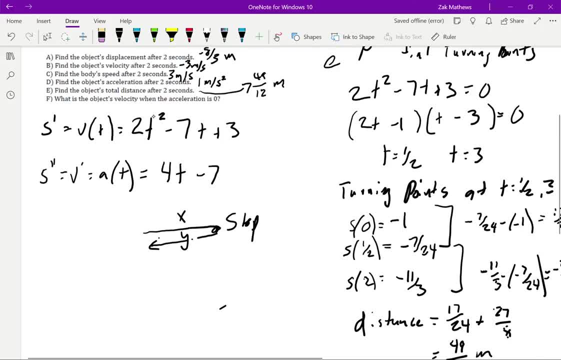 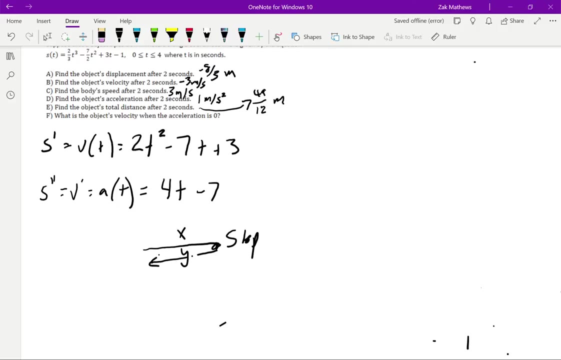 when the acceleration is equal to zero. let's clear a little bit of room here. we're not given a time here. we have to turn that time. the time we want to be using is when the acceleration is equal to zero, so we need to actually start with that. I'm gonna look for the acceleration equation which we have. I 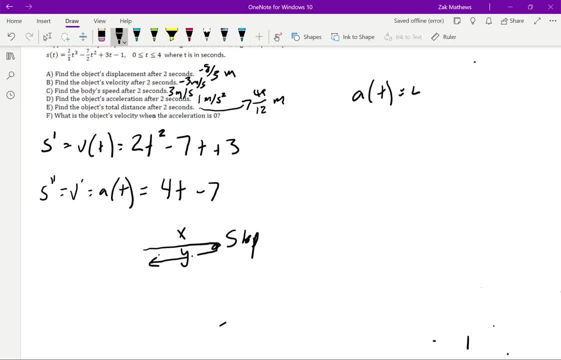 want that thing to be equal to 0, so I'm gonna set it equal to zero. I add the 7 over I'm, I divide by 4, so at t and 0, so a little b, because this\'92s the same ways you do that each one does have its own time, so we should be able to determine the time at the end of our Jagged. 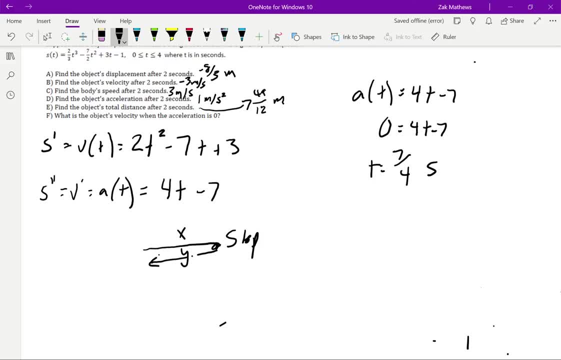 is equal to 7 fourths seconds. that is when our acceleration is zero. I wanted to know the velocity at that time, so now I'm going to take the 7 fourths, plug it into my velocity equation, which was the upper one over here. the 2 times 7 fourths squared my 7 times 7 fourths plus 3. 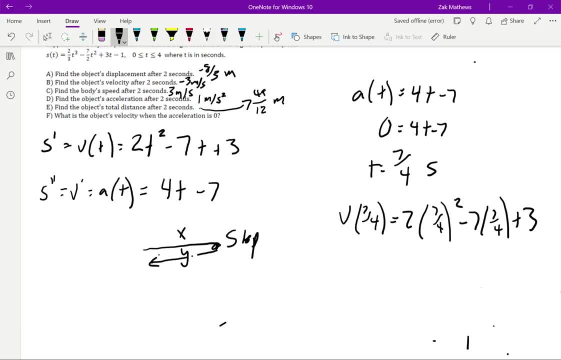 and so let me go ahead and pull out my calculator once again. 2 times the 7 fourths squared, minus 7 times 7 over 4 plus 3. when I do all that, I get the fraction negative 25 over 8, and this is a velocity. so our unit is meters per second. so that's our last part. 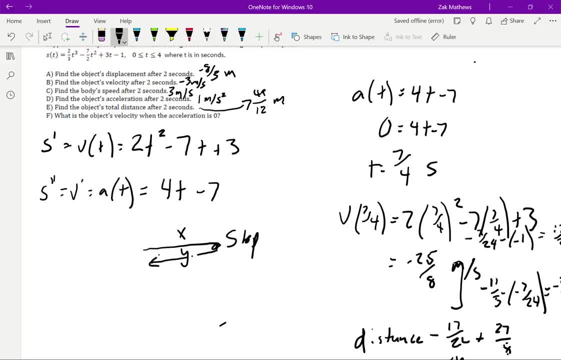 there. I don't know what happened there. It should have been a. I must have hit a wrong key. negative 25 over 8 meters per second. my work is there, it is. it's just gone scrunched in with the other stuff. all right, so there is our final answer. 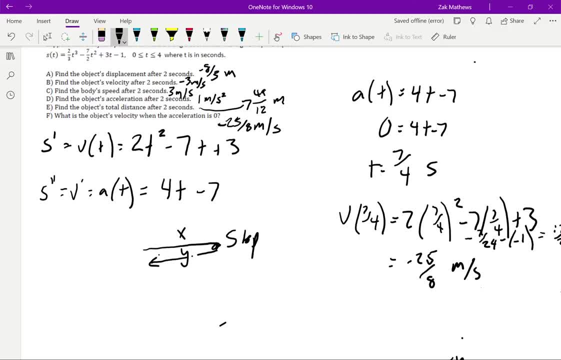 and again, because we were asked for velocity, we do want to keep that sign, the negative. so this is a good example of how we can use- we can use this speeds, we can use these accelerations, how we can use derivatives to find all of these elements. derivatives give us a rate of change. if we think about a very visual rate of change, that is the.